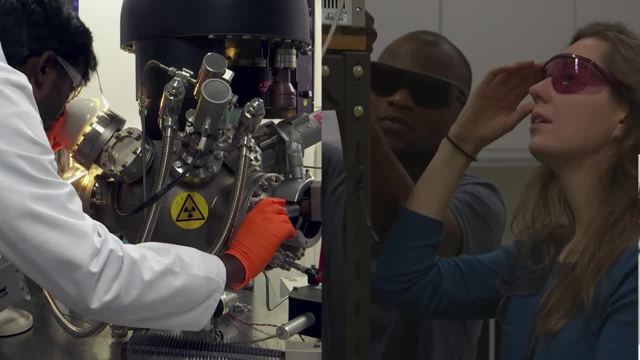 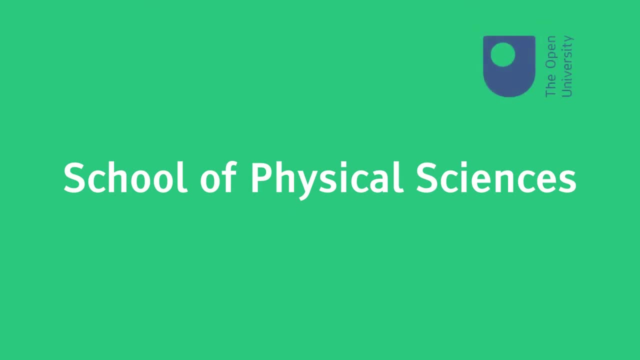 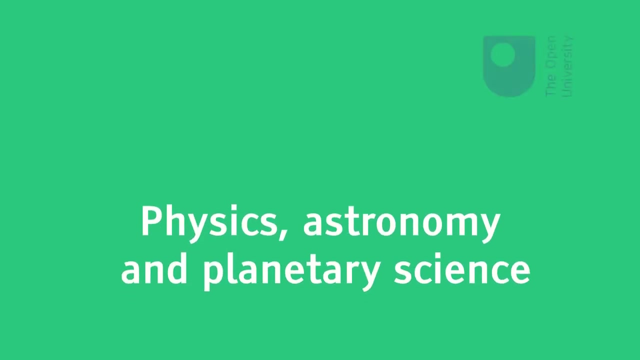 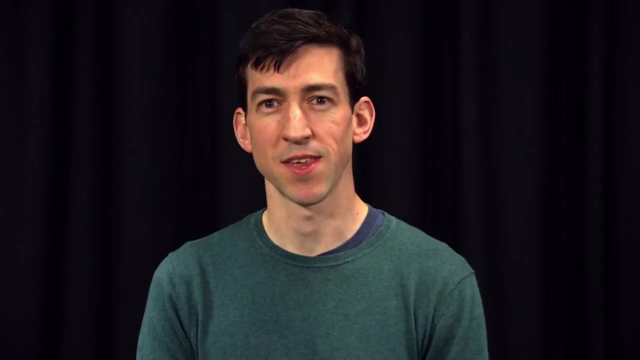 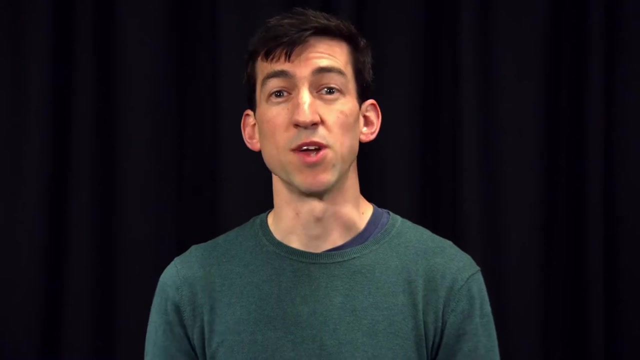 Physics, astronomy and planetary science explore the universe from the smallest to the largest scales. They address some of our most profound questions, such as: what is gravity, what is the ultimate fate of the universe, and are we alone in the universe As a physical sciences? 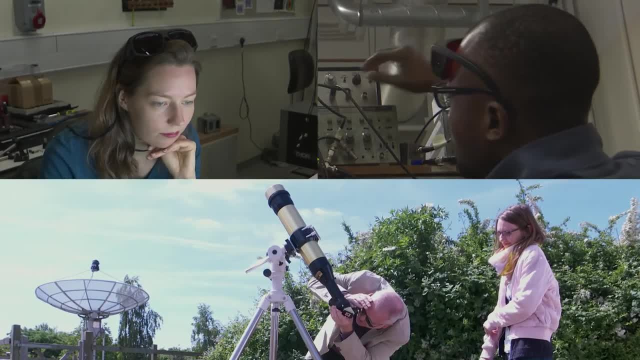 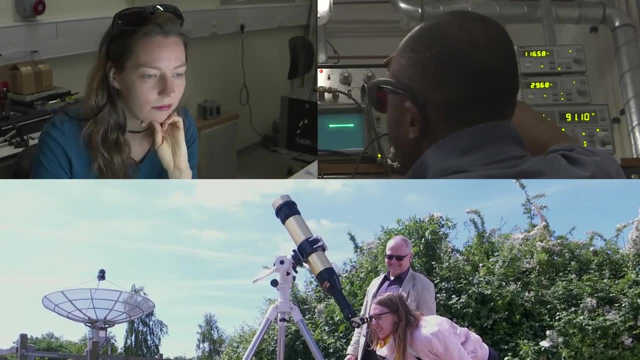 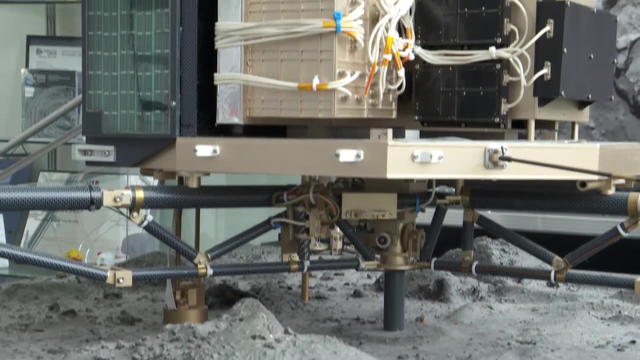 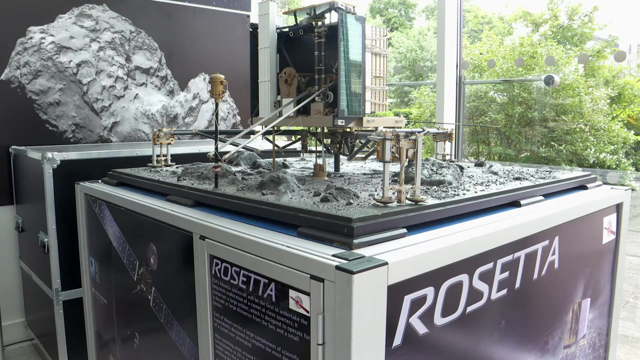 student, you will learn how to describe, analyse, test and explain physical phenomena using mathematical tools and experiments. Fundamental physics, astronomy and space exploration are among the OU's most active areas of research. For example, OU academics played a major role in the first ever landing of an analytical module on a comet in 2014 as part of the Rosetta. 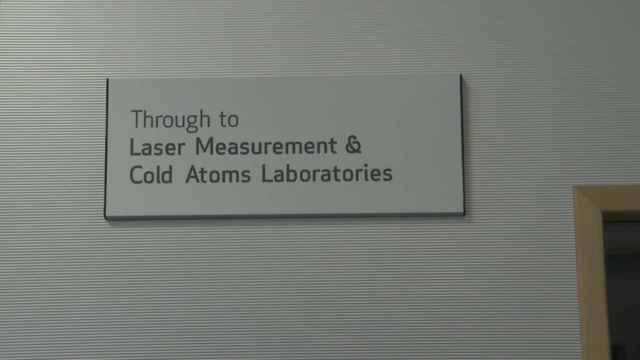 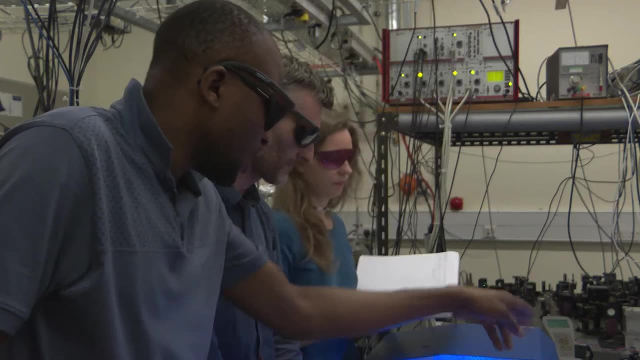 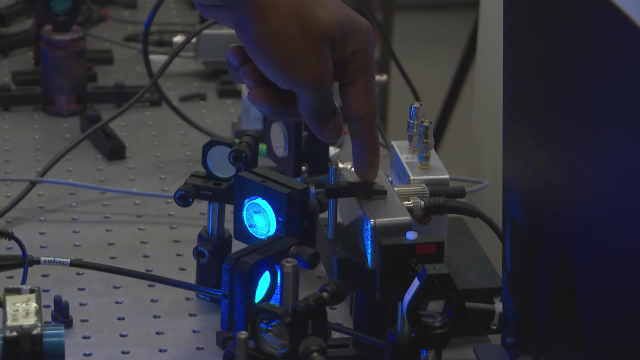 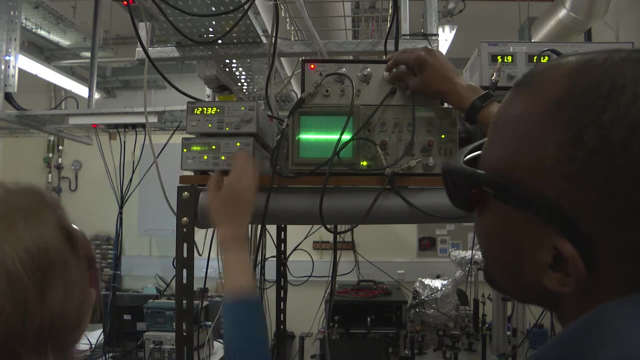 mission. Here you can see OU postgraduate students using lasers to create arrays of ultra-cold atoms to test theories linked to quantum computing. We take every opportunity to integrate our research topics and experience into our teaching. We hope this creates a dynamic learning environment as well as giving you a taste of where your studies can lead. 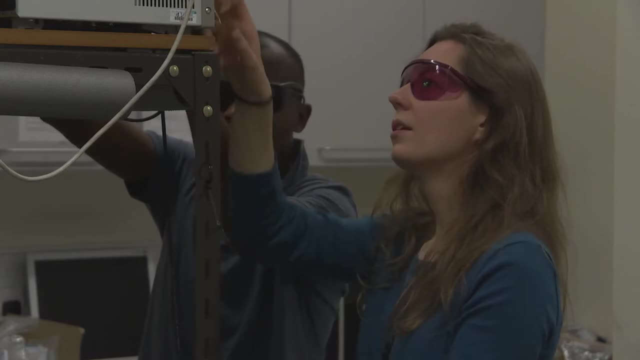 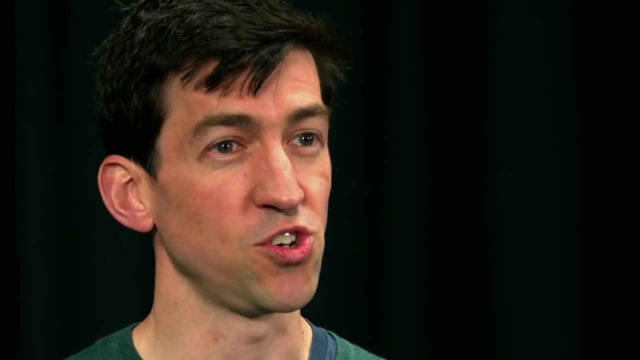 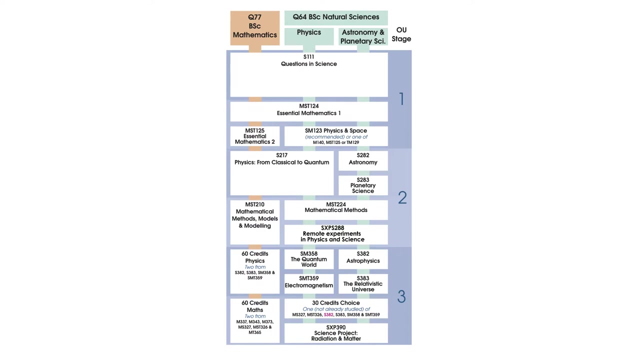 you in the future. The physics, astronomy and planetary science subject website is a new space for you to find information about our modules and qualifications, to connect with other students, tutors and academics, and to investigate future opportunities beyond your degree. In addition to the open degree and the open STEM degree, there are 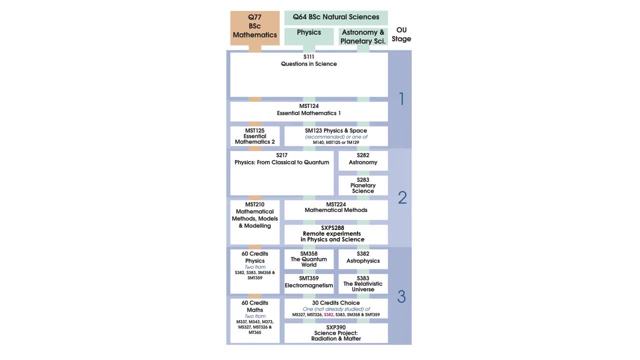 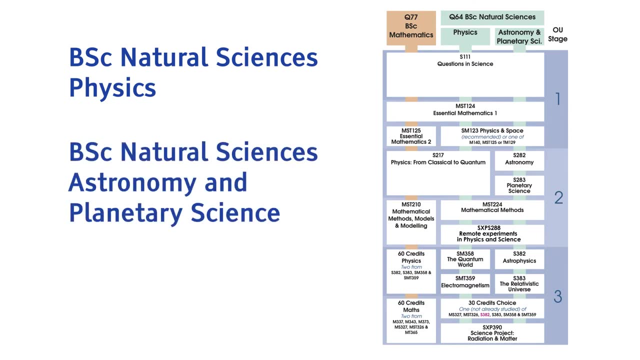 three BSc qualifications in physical sciences that you can choose at the OU. Firstly, there is natural sciences- physics. then there is natural sciences- astronomy and planetary science, and finally there is the joint degree in mathematics and physics. So now I want you to discover what it takes to become a natural character. The first: 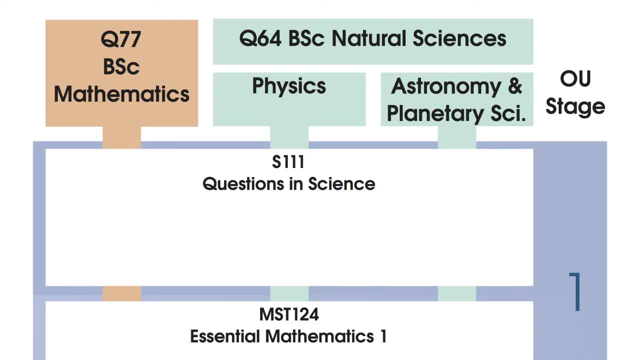 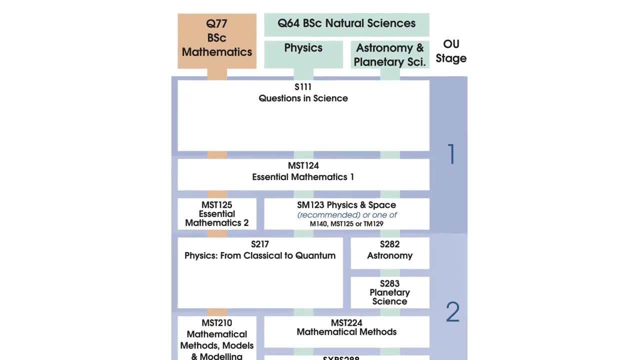 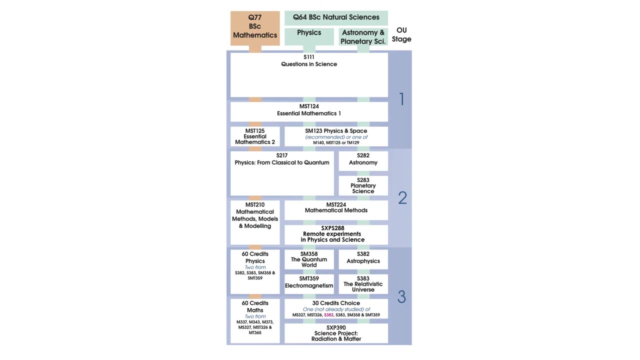 module in all three of these degrees is questions in science, which teaches concepts and skills that are valuable for all scientists. after this, there are a number of other modules that can be counted towards two or more of these degrees. This can make it straightforward for you to change your degree as your knowledge and interests develop. You can find details. 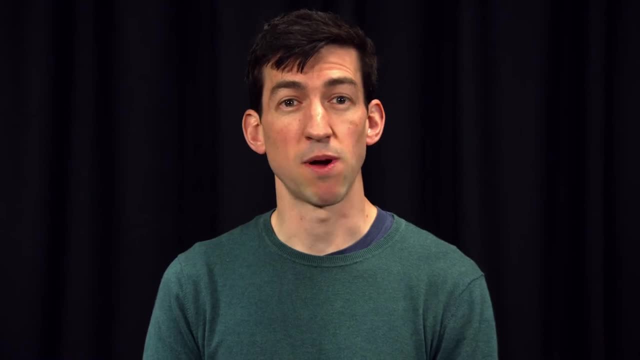 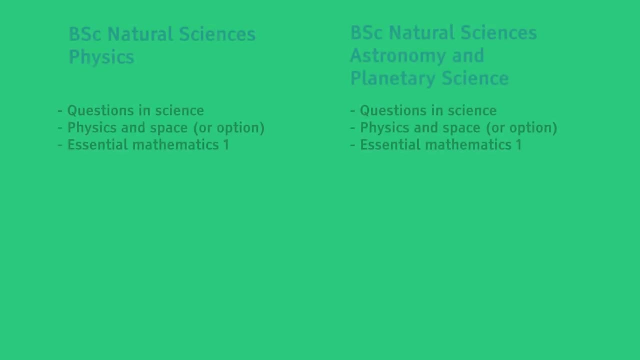 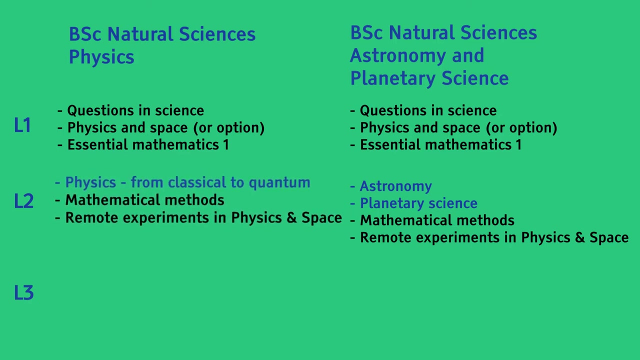 about our qualifications in the plan part of our subject website, including the combinations of Level 2 modules that enable you to claim our undergraduate certificates. The Natural Sciences- Physics BSc and Natural Sciences- Astronomy and Planetary Science BSc. only begin to diverge at Level 2.. The Physics pathway takes you to Physics from Classical 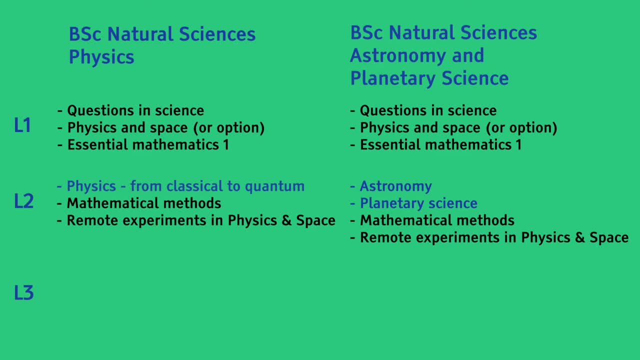 to Quantum, which gives you the broad foundation of understanding required in our Institute of Physics accredited degree. At Level 3, you will explore Quantum Physics and Electromagnetism in depth. The Astronomy and Planetary Science route features in-depth study into Astrophysics. 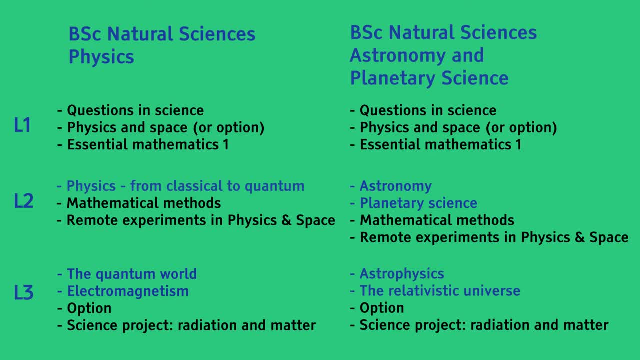 and Cosmology at Level 3.. Both degrees include an experimental module, an optional module in Level 3- Physics, Astronomy or Maths, and finish with a project module linked to a selection of cutting edge topics, such as the search for planets beyond our Solar System. 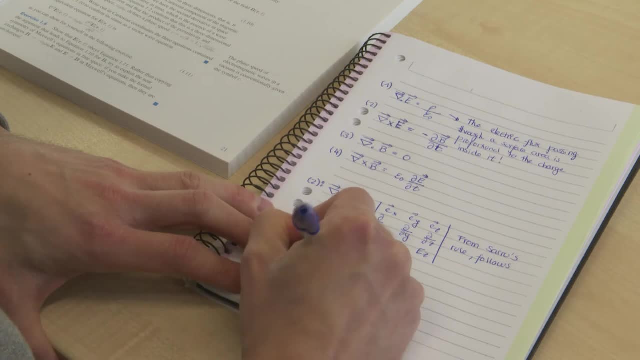 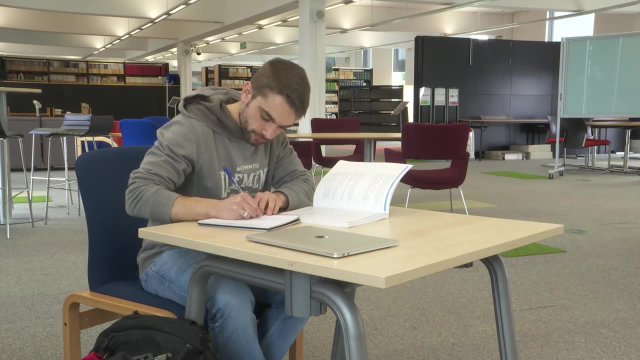 Maths is an essential tool for describing and understanding the physical world. Therefore, our Natural Sciences degrees include core Maths modules, both at Levels 1 and 2. Starting from a similar level to a high grade in GCSE Maths, these modules will enable you to develop. 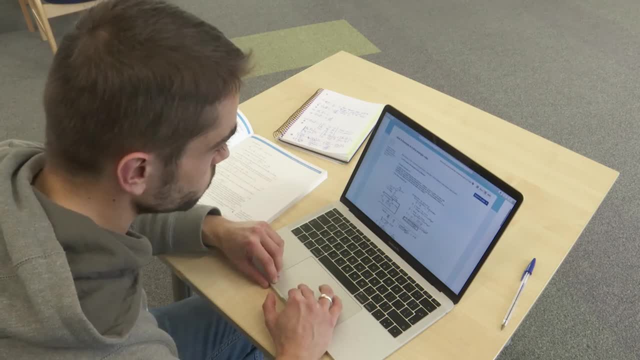 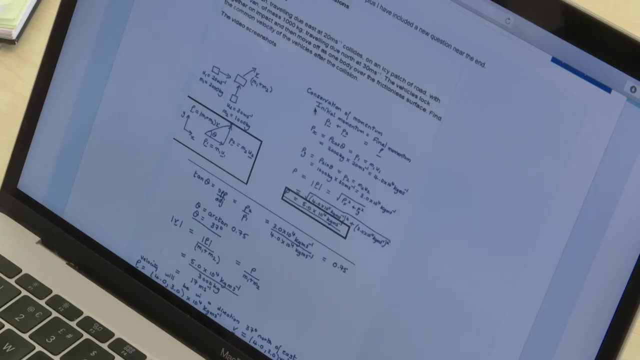 the skills and confidence in Maths that you will need to explore exciting topics such as general relativity. If you would benefit from some extra Maths preparation before getting started on a Physical Sciences degree, then the modules will be available to you at Levels 1 and 2.. 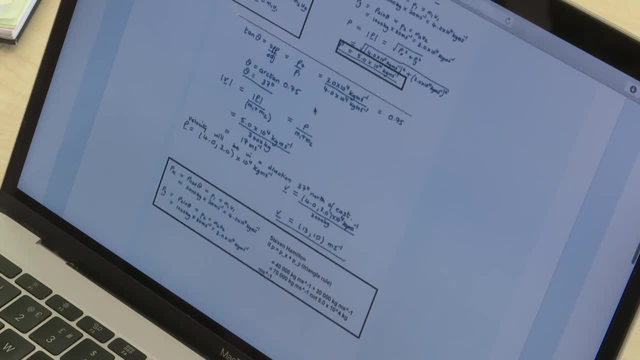 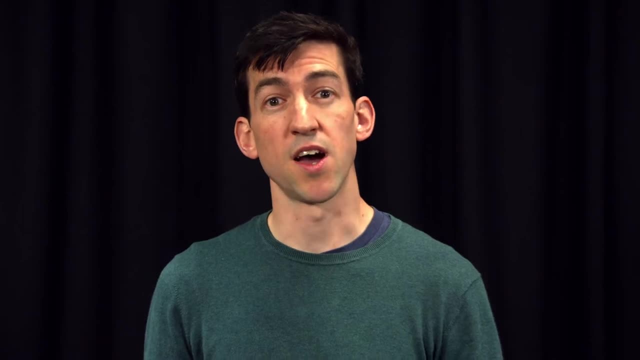 Maths is an essential tool for describing and understanding the physical world. Therefore, discovering Mathematics might be a great choice. A study advisor can help you with decisions like this. Furthermore, the Discover part of our subject website will guide you to preparation and revision activities. 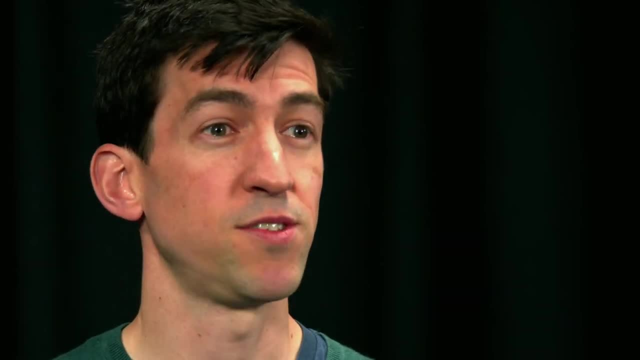 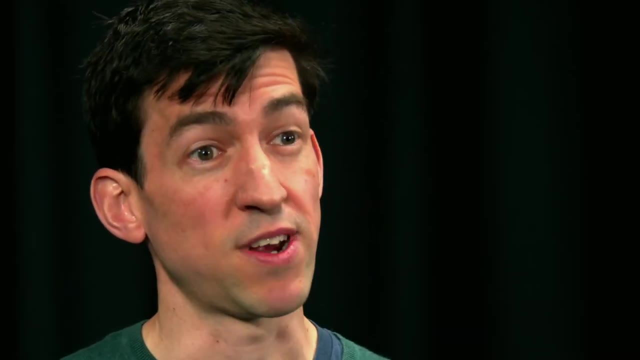 So Maths is embedded in Physics and equally, Physics is one of the most important areas of Applied Maths. There is no hard border between Theoretical Physics and Applied Maths. If your main interest in Physics is on the Theoretical side of the subject, then our 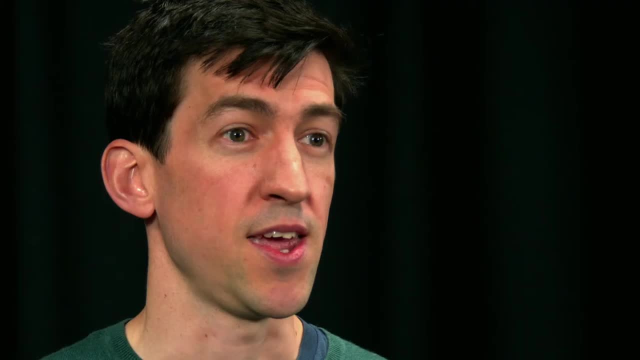 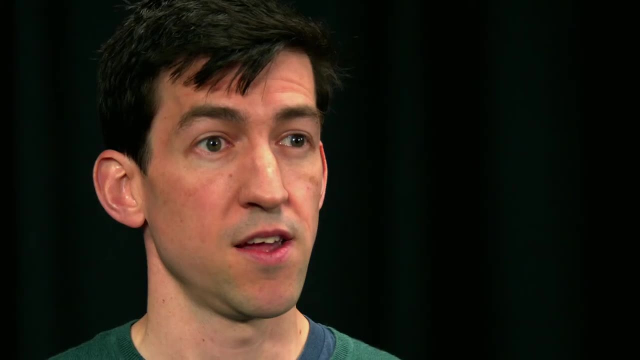 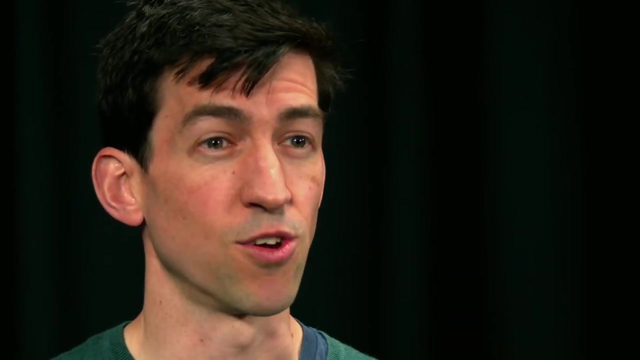 Mathematics and Physics BSc is an excellent choice. In contrast with our Natural Sciences programmes, there is no experimental work and no project module in this degree. The OU's teaching model offers great flexibility. You can work practically anywhere and you can tailor your study schedule to fit into your life. However, it also presents real 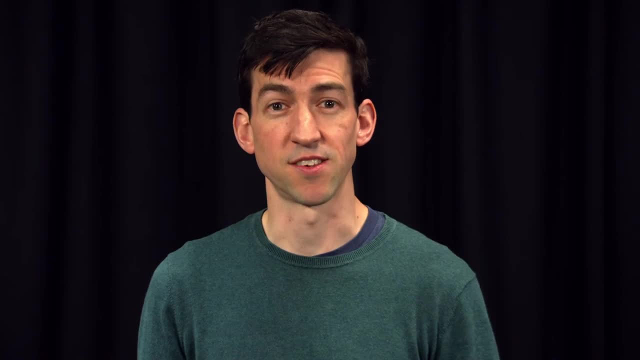 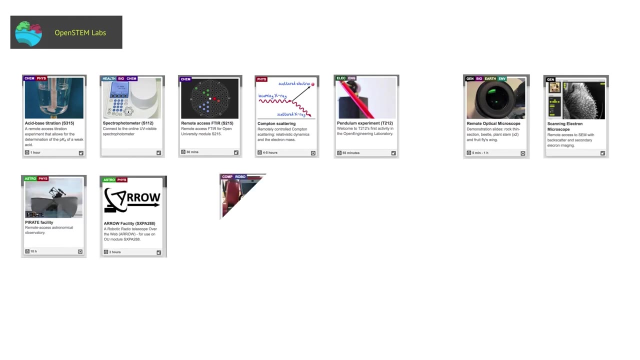 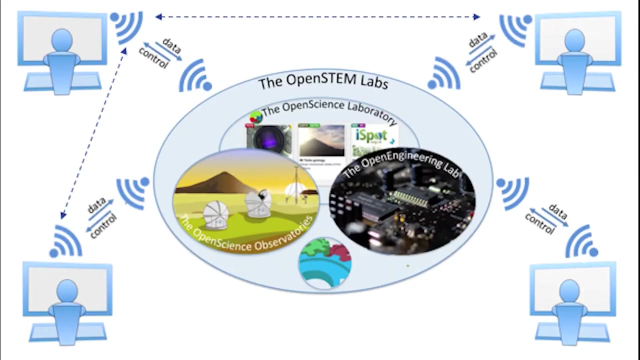 challenges in subjects with practical elements such as Physics, Astronomy and Planetary Science. In response, we have developed an award-winning suite of online practical science activities known as the Open STEM Labs. In addition to simulations and demonstrations, this includes a number of remote control systems. 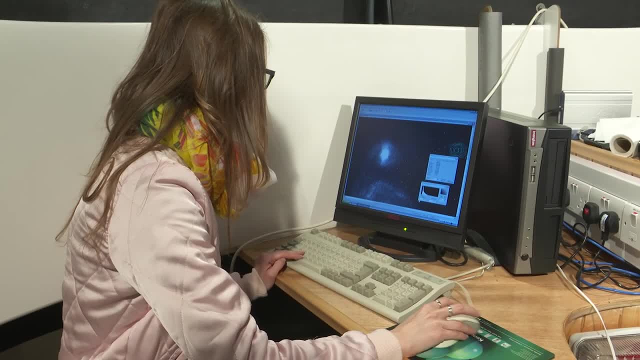 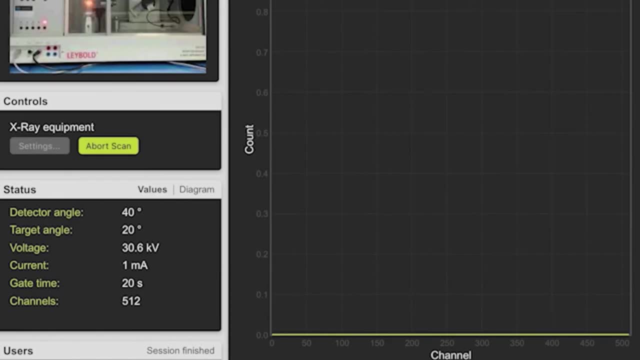 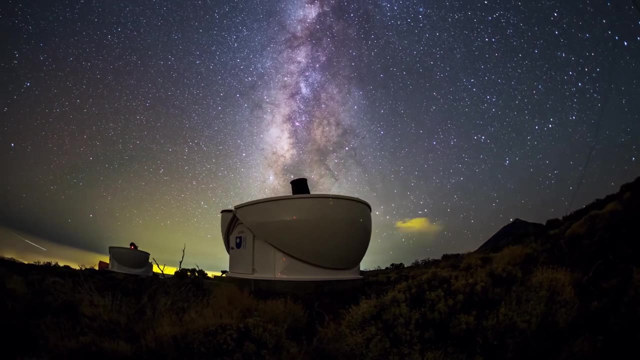 that enable students to design their own experiments, take their own data and test physical phenomena for themselves. For example, here you can see a student controlling a Compton scattering experiment, probing the so-called wave-particle duality of light. Our students also have opportunities to record astronomical images using robotic telescopes. 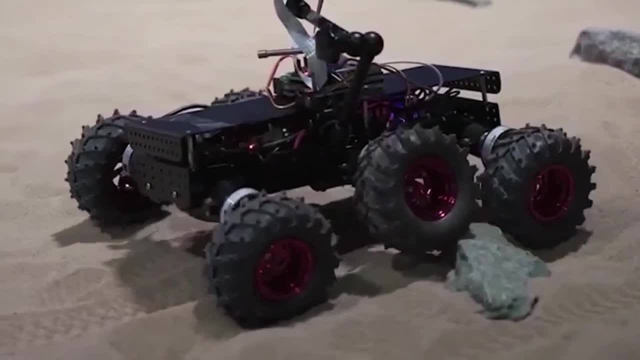 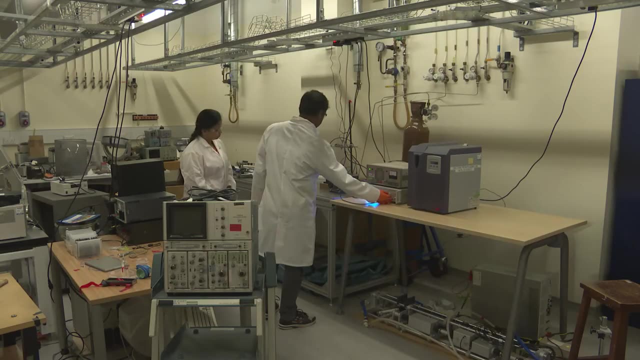 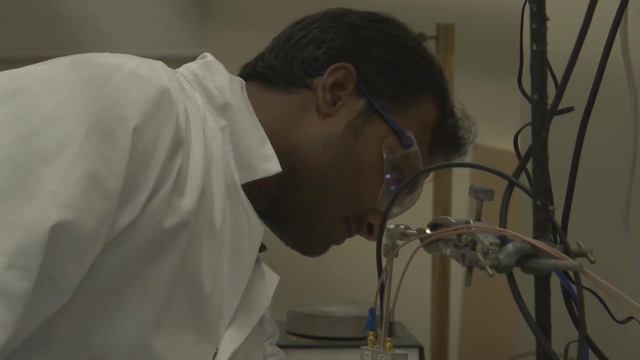 and to test a planetary rover on a Martian surface analogue built here at the OU. A degree in Physical Sciences opens a great variety of career opportunities. To give a few examples, our graduates go on to work in Medical Physics, Aerospace, Plasma Engineering and Finance. 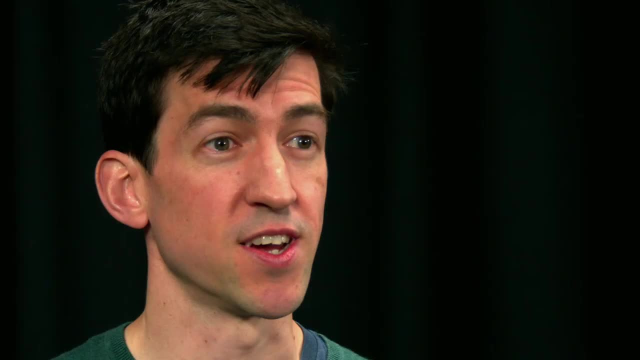 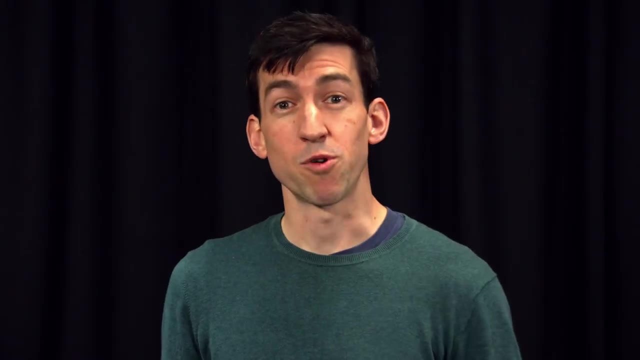 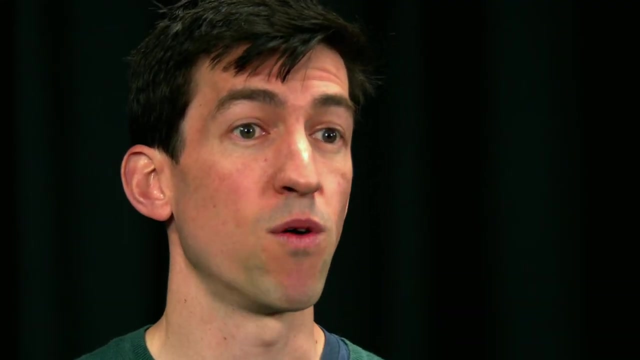 My Physics degree took me into teaching and doing experimental research at the interface between Physics and Chemistry. I study electron collisions with molecules. One of my inspirations for doing a Physics degree was reading Stephen Hawking's book A Brief History of Time. I was fascinated by the ways in which classical Physics concepts can break down when you look. 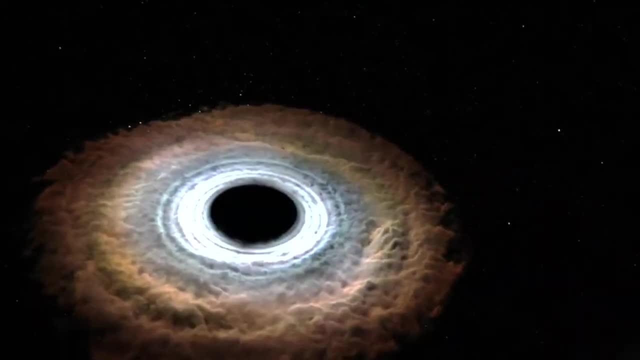 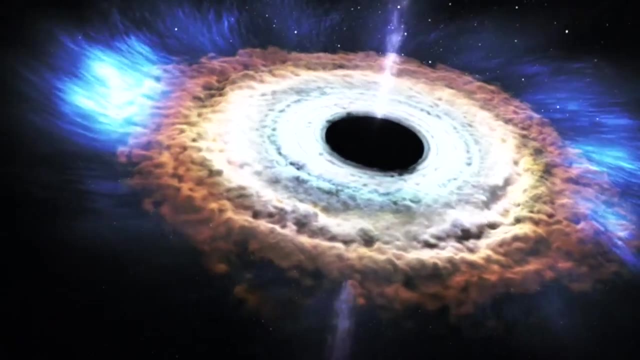 outside our familiar environment. Black holes, one of Hawking's main interests, are an extreme case. But even the humble electron turns out to be very strange. For example, it has a fixed angular momentum. Nothing can be done to stop, speed up or slow. 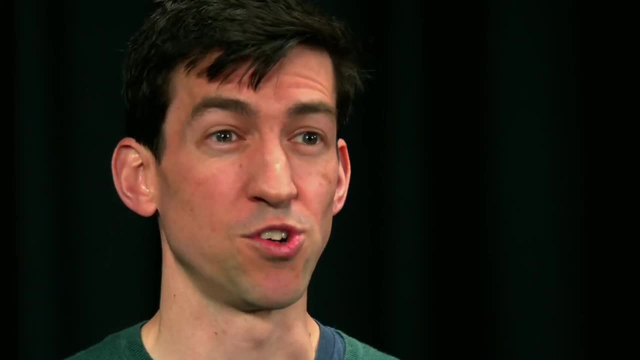 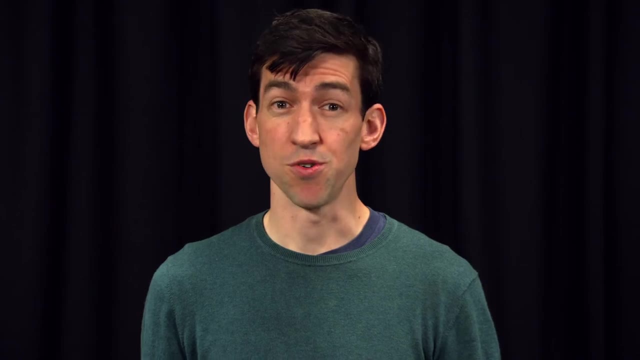 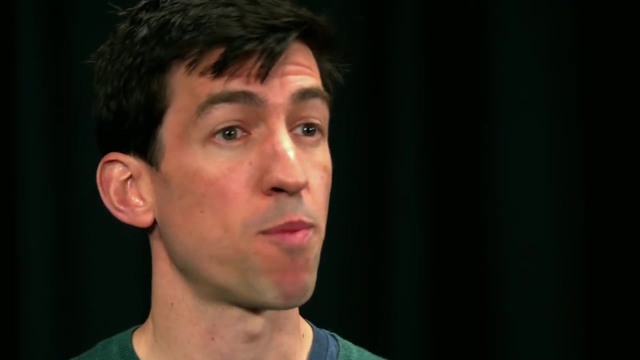 down this so-called spin. This is deeply counter-intuitive, but when you study Physics at Level 2 and Level 3, you'll see not only that it is manifestly true, but also that it has huge implications. It's no exaggeration to say that we can't understand Chemistry without properly accounting for. 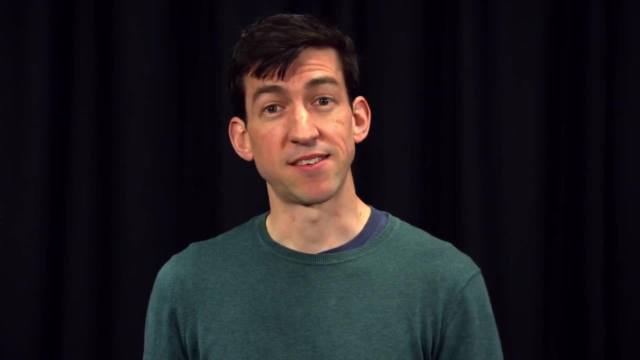 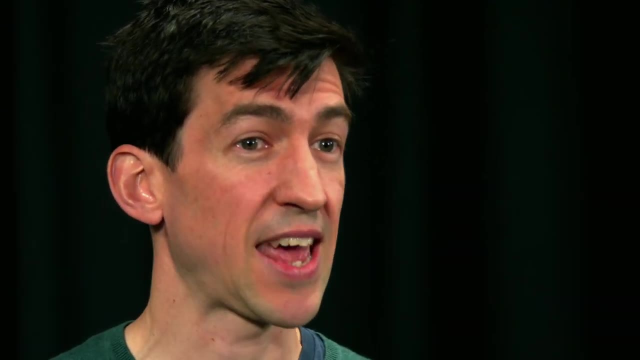 electron spin. Over the 20 years or so that I've been studying and working, Physics has never stopped surprising and challenging me. My colleagues in Astronomy and Planetary Science will tell you the same about their fast-moving fields. We hope we will find learning about the physical world at the OU as exciting and rewarding. as we do.